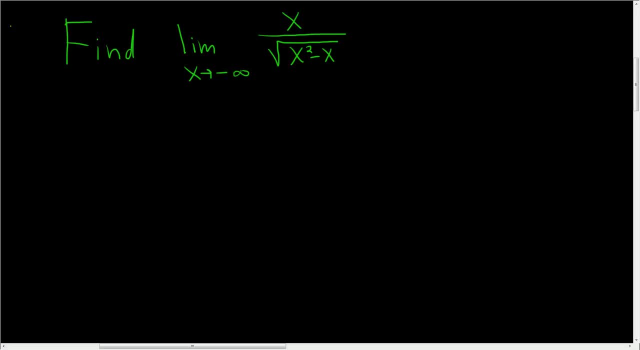 Okay. so we have to find this limit. Let's do it two ways. Let's do it the quick way and the regular way, the way you're supposed to do it. So the quick way, The quick way, will give us some insight into what's going on Before we do it the quick way. you should note that the square root of x, squared, is equal to the absolute value of x, which is a piecewise function. This is equal to x if x is greater than or equal to zero, And the opposite of x if x is less than zero. So 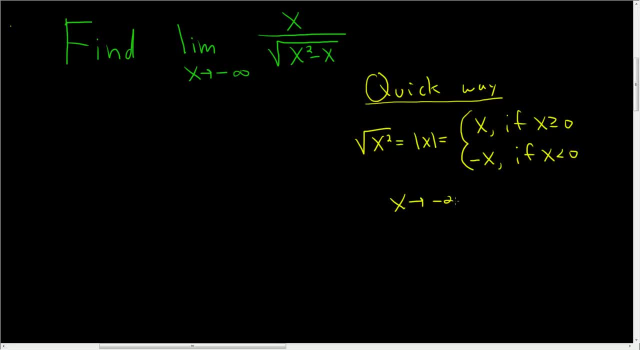 in our problem, x is approaching negative infinity. That means that x is less than zero. So the square root of x squared is the absolute value of x, which is equal to negative x. Super, super useful stuff here. This is key. It's like you cannot avoid this in calculus, Not just this problem, but there are so many problems where this is the. this is the key to doing the entire problem. So if we do it the fast way, we can ignore the. 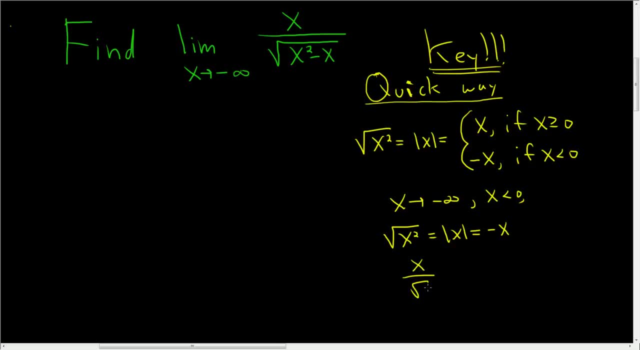 x, And so we really have x over the square root of x squared, which is x over the absolute value of x, which is x over negative x, which is negative one. And as x approaches negative infinity, this approaches negative one as x approaches negative infinity. So this should give you some insight into how to do the problem the correct way, you know, showing all the work. So solution. So we'll take the limit As x approaches negative. 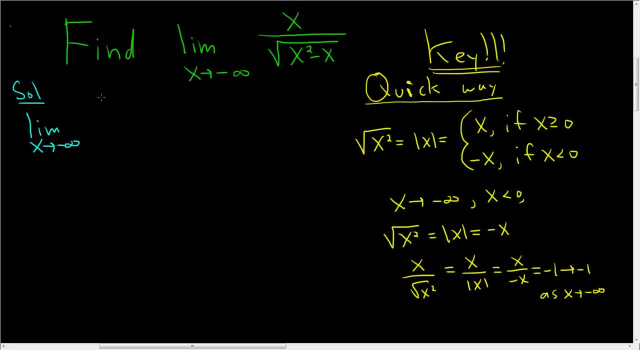 infinity, And we'll divide by the square root of x squared. in the numerator, we'll have x over the square root of x squared, And in the denominator, we'll have the square root of x squared, minus x over the square root of x squared. Okay, so we're doing the same thing we did in the previous videos, except now we're dividing by the square root of x squared, So this is equal to the limit. 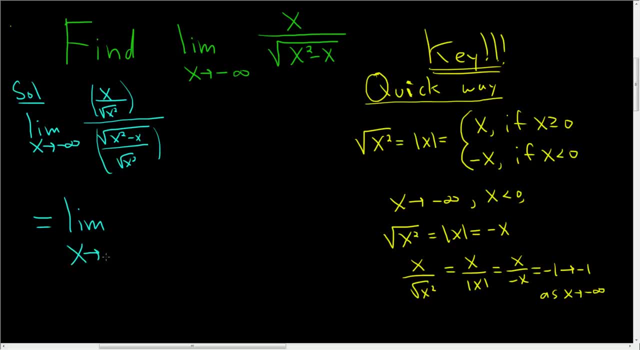 as x approaches negative infinity. Now in this problem the square root of x squared is equal to negative x, because x is approaching negative infinity. So we can write this piece as x over negative x, But x over negative x, that's just negative 1.. So the